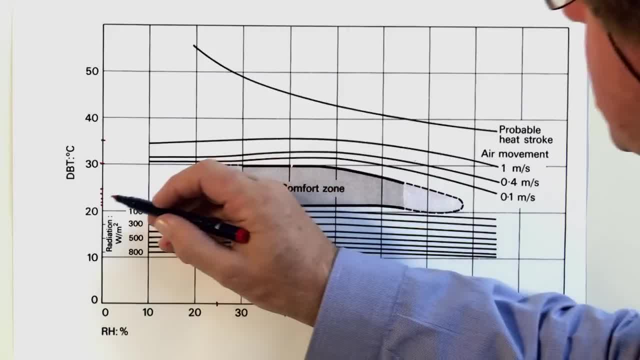 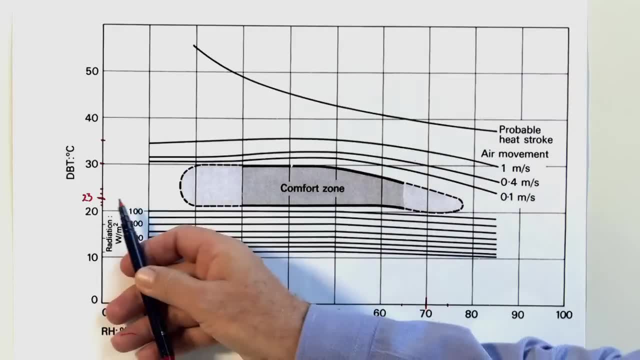 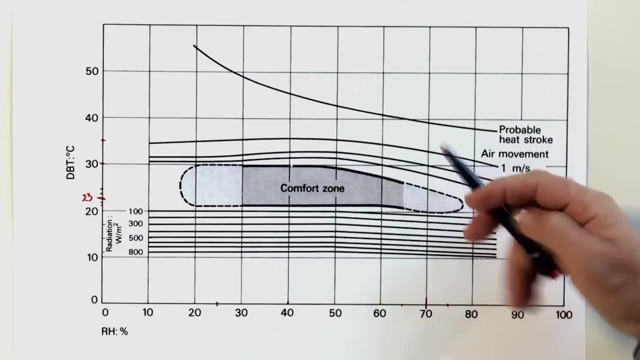 The dry bulb temperature was 23 degrees. So 23 degrees plots about here. We move across and we intersect with the 70 percent relative humidity. This is going to bring us to a point about here which tells us that we're pretty close to the comfort zone. 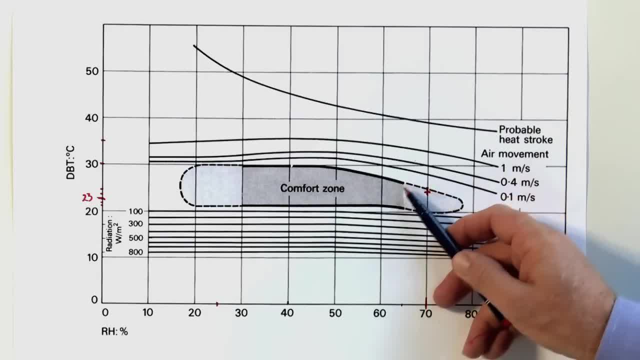 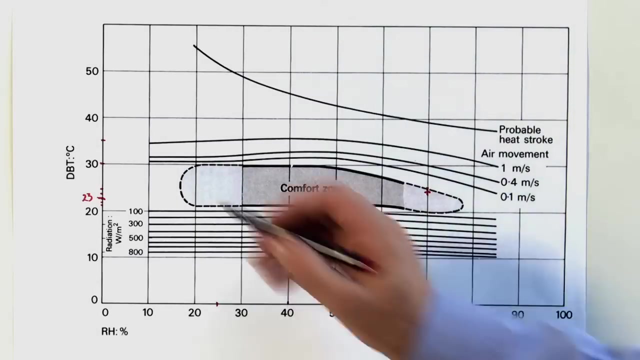 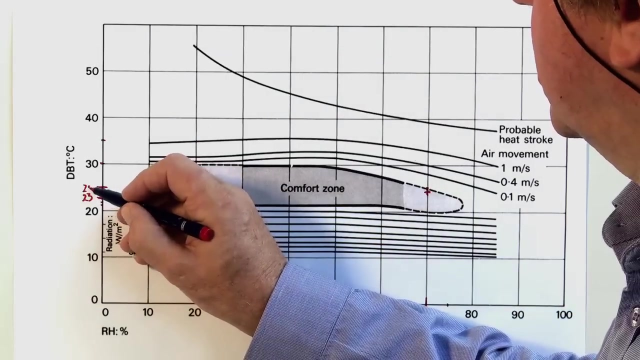 and it's a little bit out of what we would accept. This dash, dash dash line indicates that it's borderline. The next example that we looked at was 65% relative humidity and we looked at 25% dry bulb temperature. So the 25% plots here We then plot across intersecting with 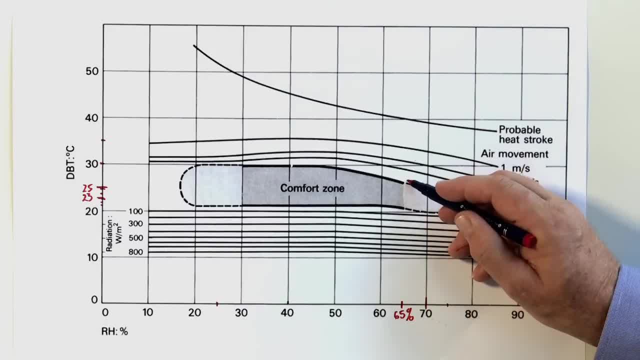 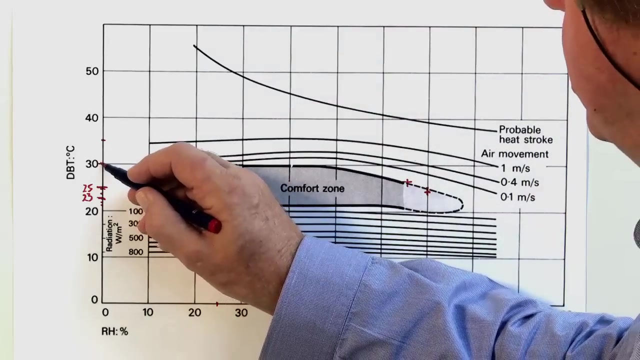 the 65%, and again we're right on the border of the comfort zone. The next example we looked at was 40% relative humidity. In this case we were looking at a dry bulb temperature of 30 degrees Moving across. 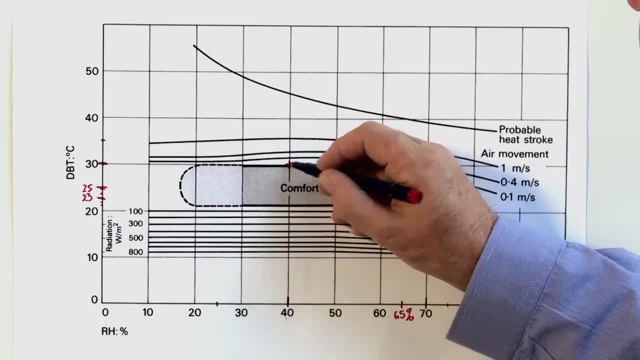 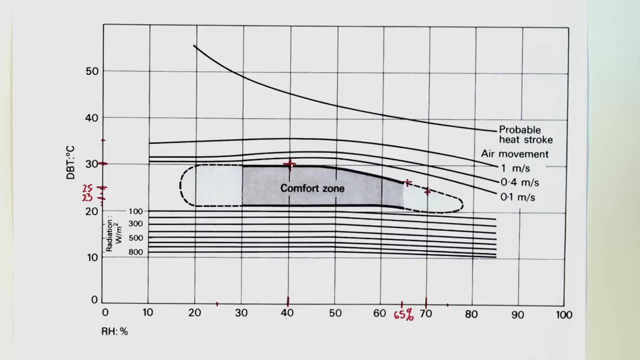 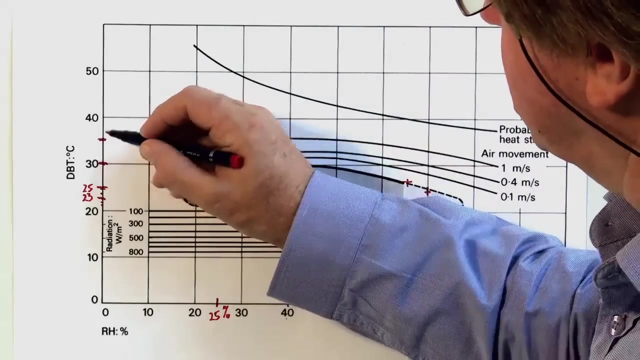 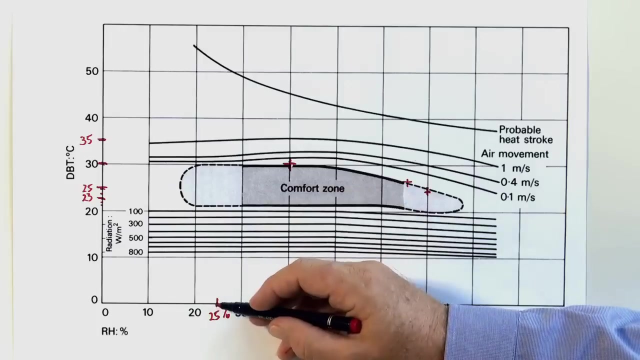 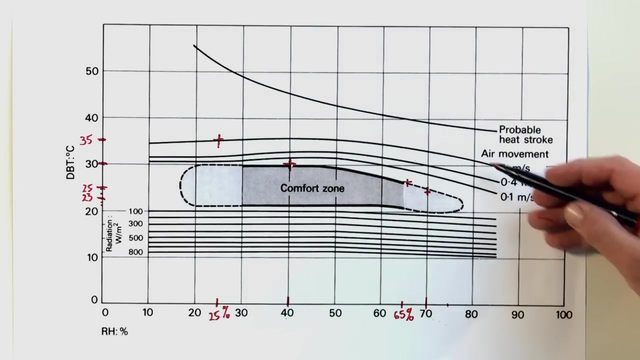 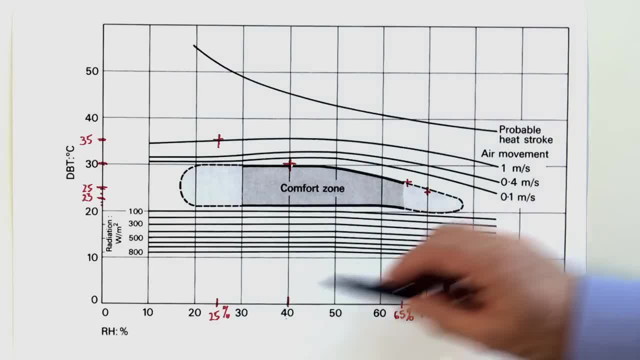 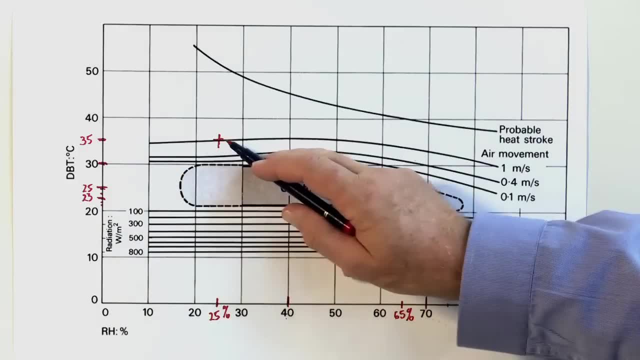 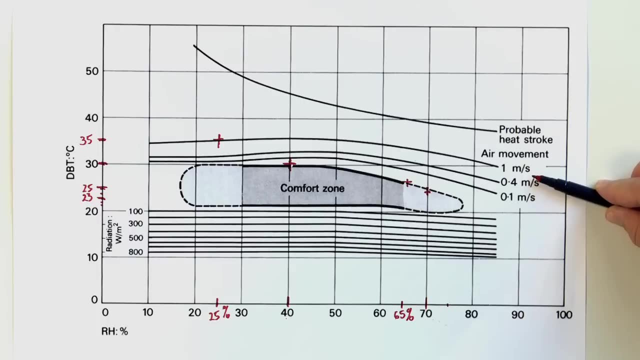 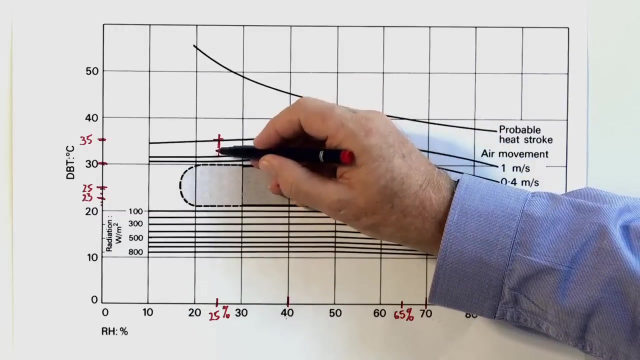 temperature, the comfort zone, And so in the case here of 25 degrees relative humidity and 35 degrees dry bulb temperature, by introducing air movement at one metre per second, we can pull the temperature down to something that would simulate a comfortable zone. 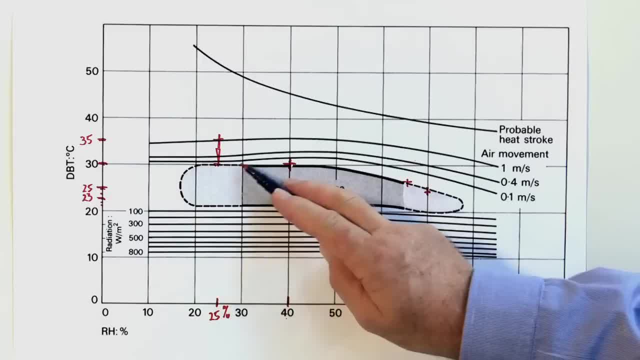 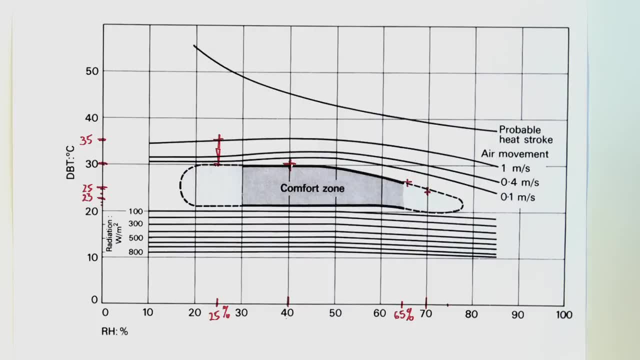 The trouble is, here we are again in this dash dash dash line which is borderline for human comfort. The beauty of the bio-climactic chart is we can see how we can use air movement to pull the temperature down If we have 0.1 metres per second. 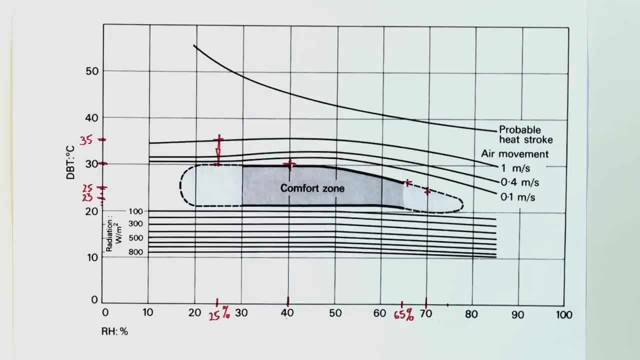 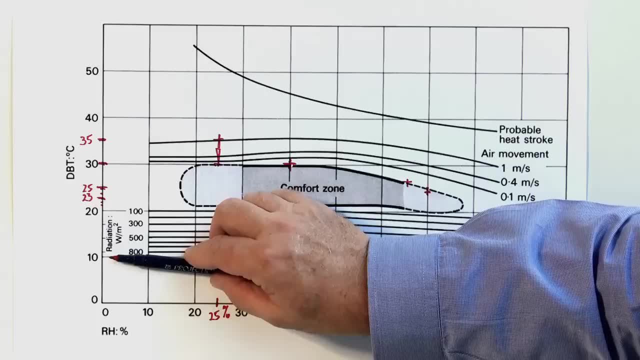 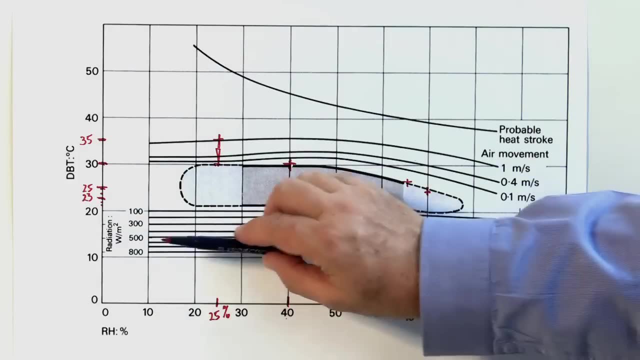 we can pull it down into the comfort zone. The other beauty of the bio-climactic chart is it tells us, when we have temperatures down to 10 degrees Celsius, through to 20 degrees Celsius, how many watts per square metre need to be introduced.